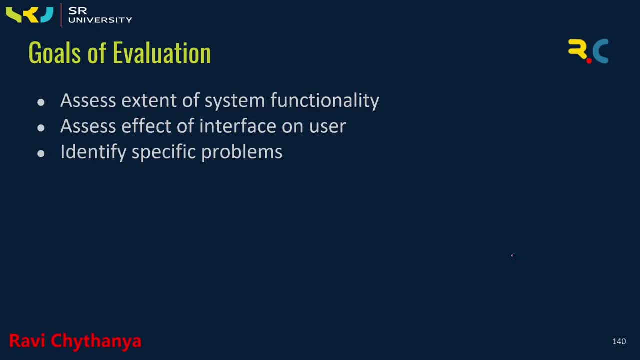 evaluation are: first one, it is going to evaluate or assess the extent of the design, And then we are going to assess the extent of the system functionality. And the next one, it is going to assess the effect of the interface on the user in terms of the visibility, the audibility or in. 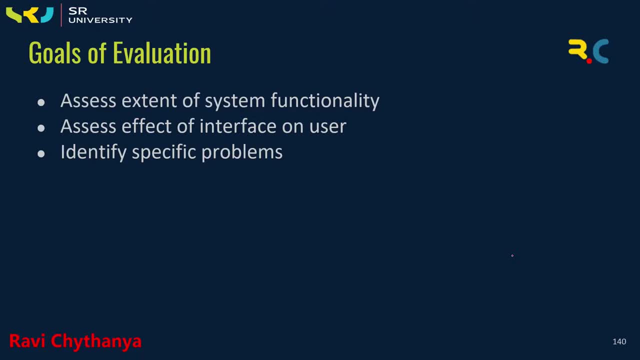 terms of the usability. we are going to assess that thing And then we this assessment. the evaluation is going to identify the problems in the specific areas like design- okay, the user in terms of the screen. design in terms of the layouts and in terms of the things- okay, whatever. 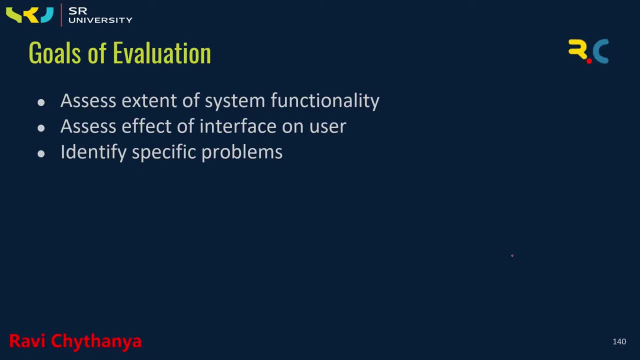 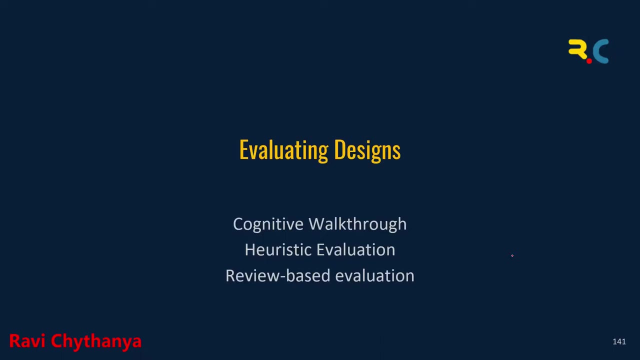 we have. okay, whatever we need to consider all the things, all the considerations are going to be tested and evaluated, And there we are going to identify some specific problems. Okay, so these are the goals of the evaluation, And then we are going to learn about the evaluating designs. Okay, 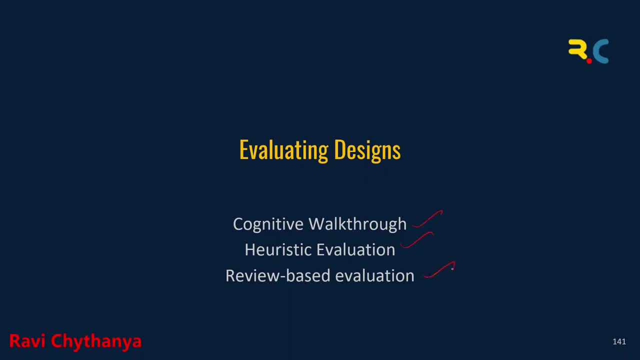 here we have discussing about the three types of the three evaluating device. the first one is cognitive walkthrough, The second one is heuristic evaluation And the third one is a review based evaluation. The cognitive walkthrough is nothing, but it is going to evaluate the design and how. 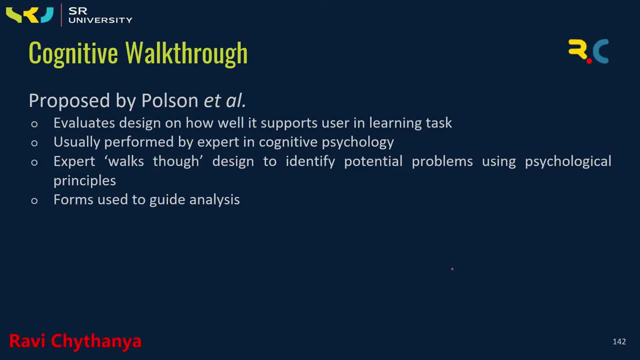 well, it supports the user in the learnability of the task view which you have designed or developed. Okay, so, and then it is going to be performed by the. it is going to be performed. the cognitive walkthrough is going to be performed by the experts. 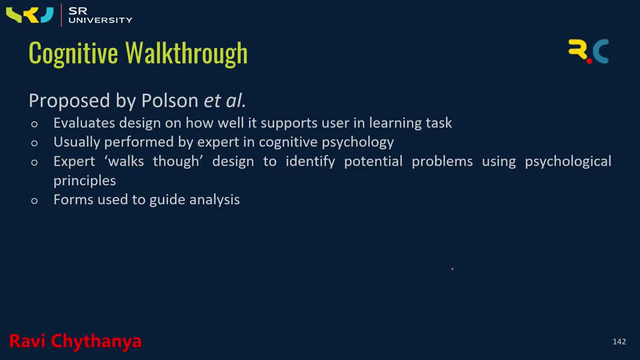 who are in the cognitive psychology, who are experts in the cognitive psychology. Actually, this cognitive walkthrough was proposed by the Paulson. Okay, so he has told that he has proposed that the whatever the cognitive walkthrough- designing- sorry, evaluating, design- okay. 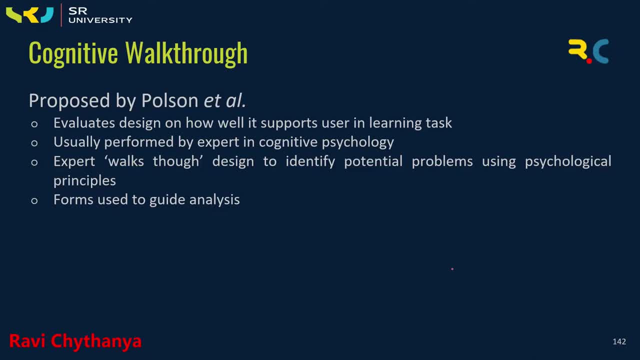 so that has to be done. that has to be done in the supervision of the experts in the cognitive psychology And the expert is going to walk through the design to identify the potential problems using psychological principles. That's why we are calling it as walkthrough. Okay, and here we are using the psychological principles. that that 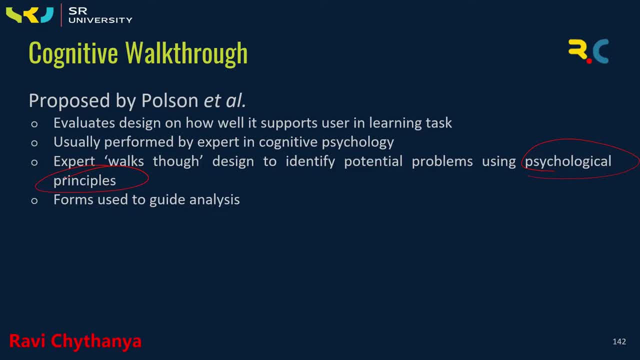 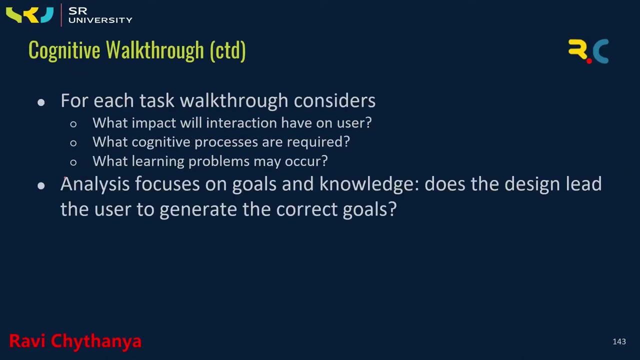 that because it becomes the cognitive walkthrough, And this cognitive walkthrough forms, use it to guide the analysis of the analysis of the system which you have developed. Okay, so here, for each task walkthrough, considers okay, for every task, the walkthrough, the cognitive. 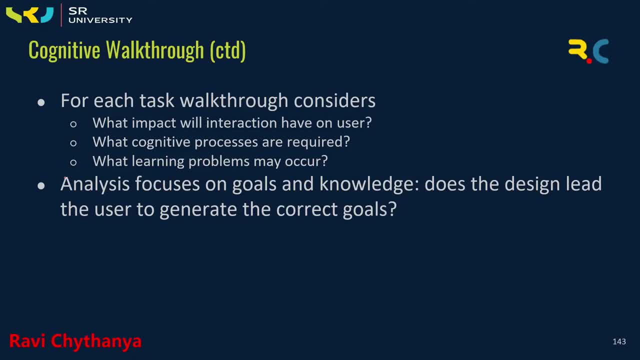 the psychological principles. according to the psychological principles, the walkthrough considers: what impact will interaction have on user And what is the cognitive process? What are the cognitive processes which are required to confirm, which are required to evaluate the design and what learning problems may occur while learning the design? 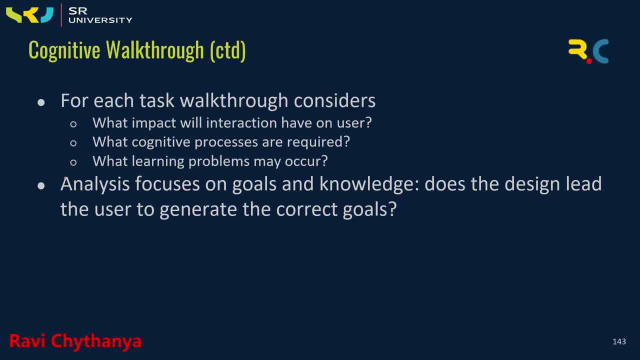 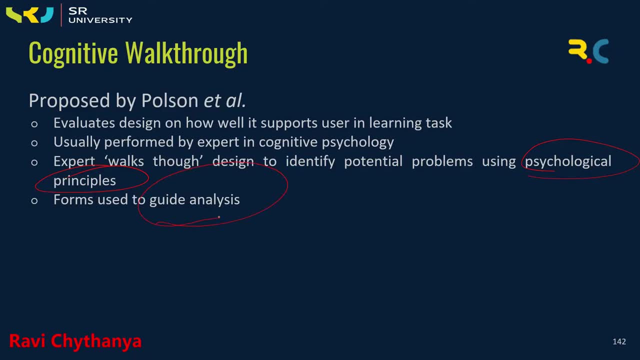 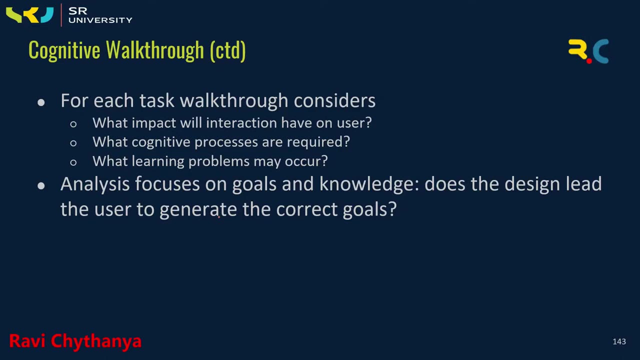 You have developed and analysis, Okay. so after completion of the thing, okay we are going to. we are going to analysis, analyze the system. this analyzing focus on the goals and knowledge that the design lead the user to generate the correct goals or not. The goals are nothing but okay. 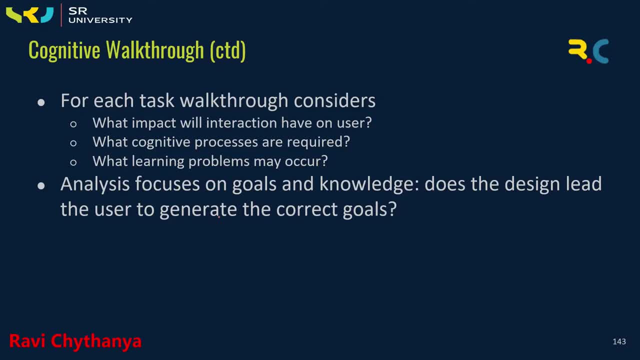 so if I'm going to, if I, if I'm developing an application for some specific person of specific reason, specific purpose, okay, then that specific person purpose has been achieved by the, achieved by the design or not, is going to be, this is going to be decided or it is going to be analyzed through. 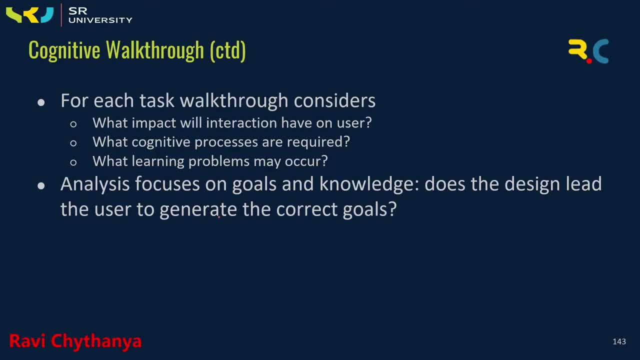 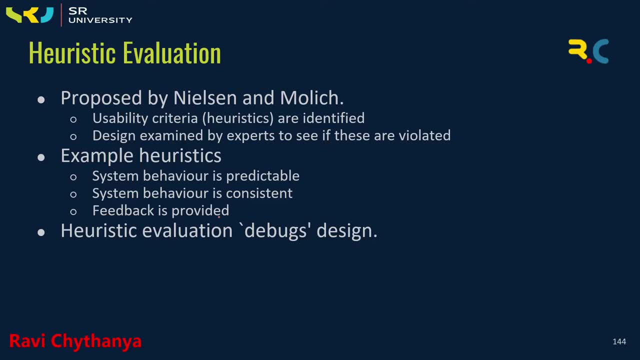 the cognitive walkthrough. And the next thing is we are going to discuss about the heuristic evaluation And this was proposed by Nielsen and Mollich And the criteria. actually, it is going to hear the heuristic is nothing but it is a criteria and the usability criteria is going to be identified before examining by the experts and the design. 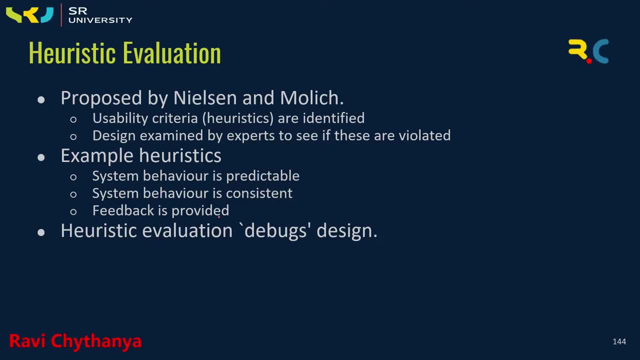 examined by experts to see if these are the criteria are violated. Whatever the usability criteria, first of all, okay, so whatever. if I'm going to have one application, okay, so that application is used for reservation of the railways, okay, then, first I need to identify the usability criteria And then 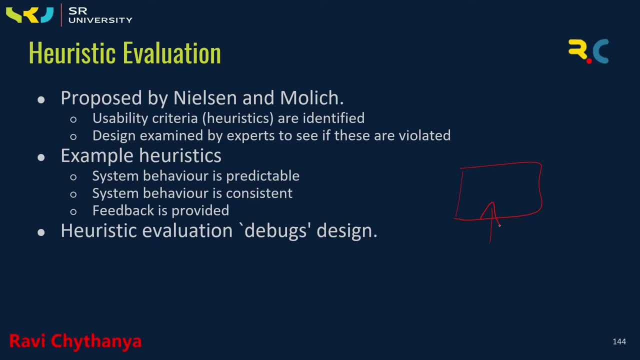 the experts are going to, as this, examine the design by seeing if those criteria- whatever the criteria you have, usability criteria you have identified that are violated or not. if they are violated, then that design is not according to the according to the requirements, okay, and the? 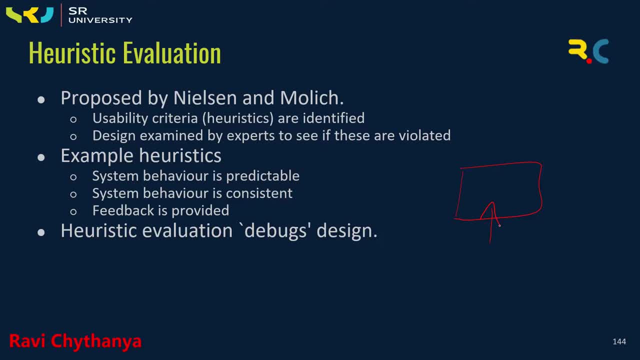 example, criteria are: system behavior is predictable, system behavior is consistent and the feedback has been provided. If I have designed one application for the railway reservation system, for example, and once I have done with my reservation, okay, it has to give me some feedback that you are, you are registration. 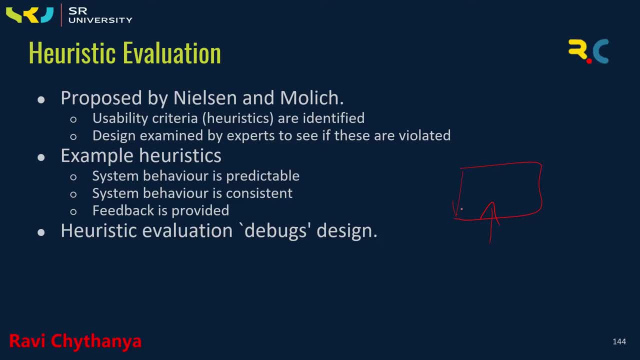 your reservation has completed successfully And here is your ticket And this is your waiting list or this is your confirmed ticket numbers And this is your confirm the seatbelt bed number and all these things has to be given by the system. if they were not given defined or if they were not given, given back the 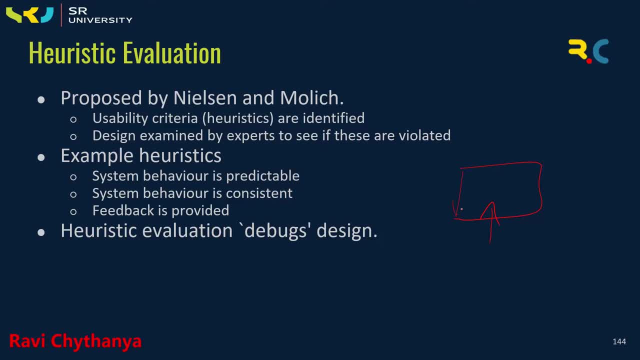 feedback is not provided, then that system is useless actually, because I have selected the better than bets, bets in the rail train coach, Okay, and then I have paid amount, okay, And then it has to give me feedback that the payment is valid. It will give some feedback. it will give some feedback. 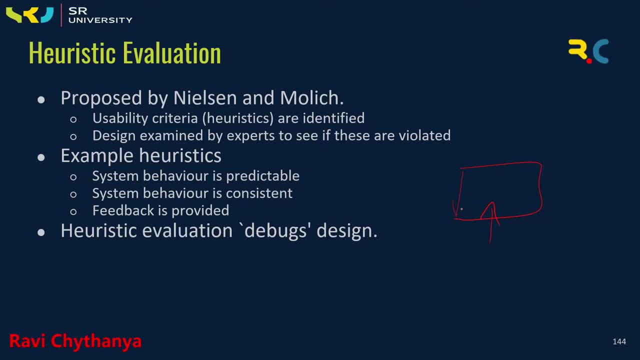 was successfully and the seats were reserved for you successfully. the number of seats reserved for you is two and the numbers, the seat numbers, are s11. in s11 coach it is 14 and 50.. okay, so the heuristic evolution debugs the design. actually, this criteria based evaluation is going to. 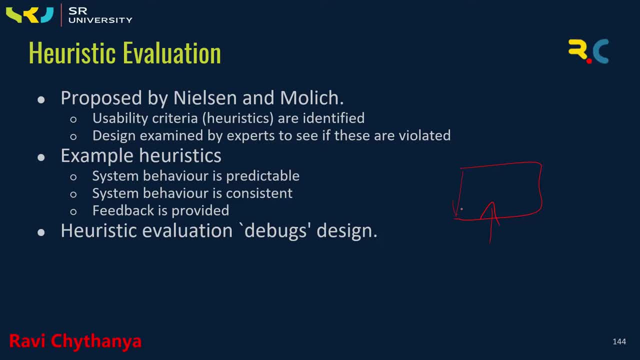 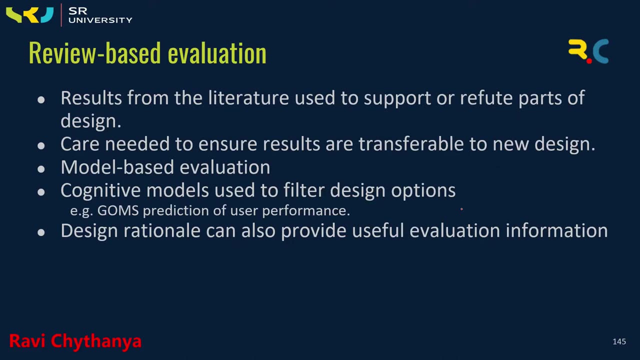 debugs the design, it is going to check for the errors, or the behavior is correct or not. everything is going to be checked or examined by the heuristic evaluation. and the next one is review based evaluation. here the name itself saying the review. okay, so the results from. 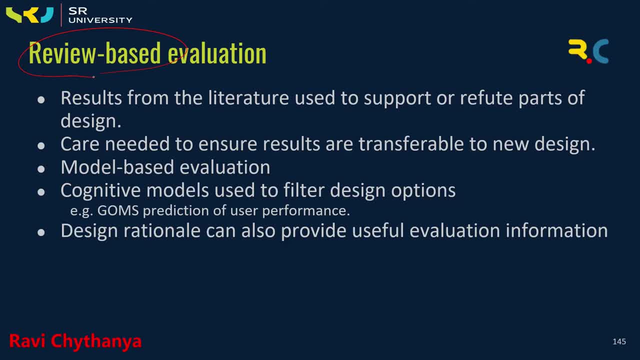 the literature used to support or refute parts of design. so you are going to take the reviews. you are going to take the reviews and then this is going to how this is going to evaluate for the designs, frosts and this is actually a model based evaluation and the cognitive models used to 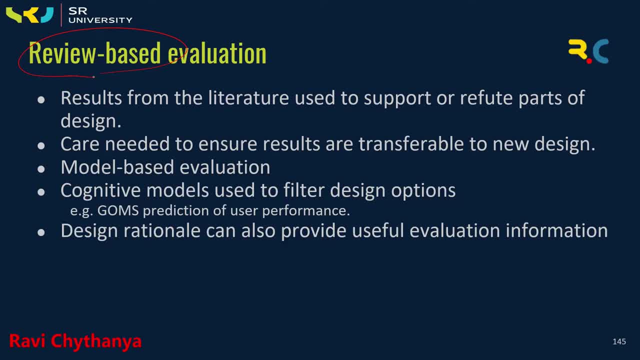 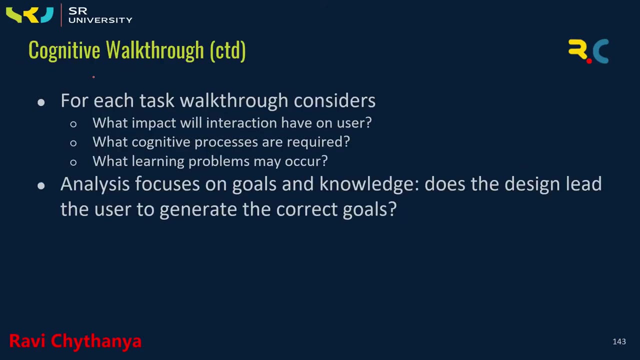 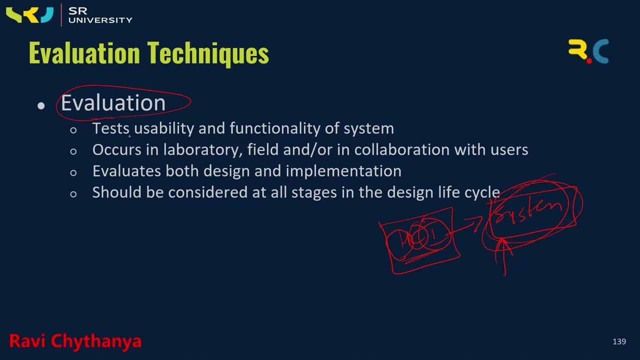 filter, design options, the goms prediction of user performance and the design rational can also provide useful evaluation information. this is regarding the review based evaluation and the next thing is application through user participation. okay, is this okay? in the first slide, the evaluation techniques. what has been by evaluation? okay, so here, the test of the usability test and 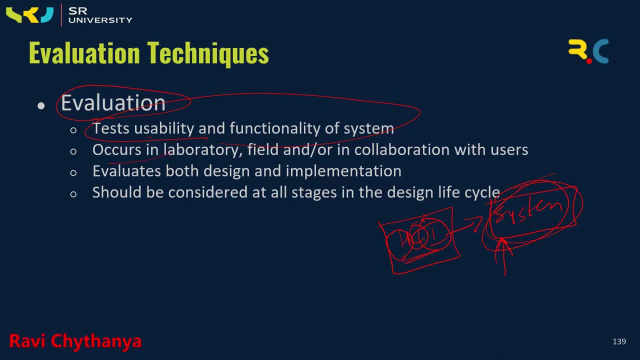 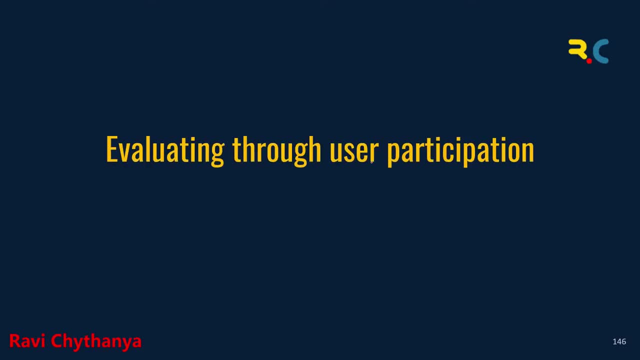 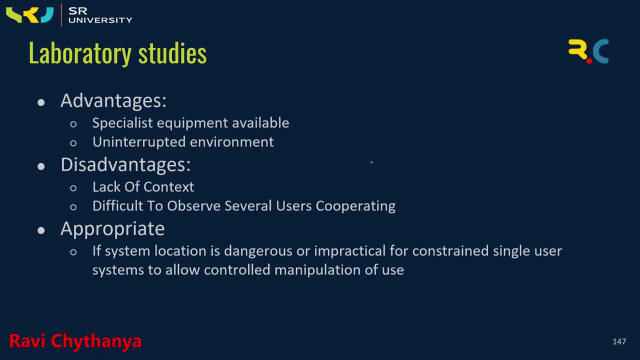 test the usability and functionality of system. that can be done by the designs, evaluation designs, and then you are going to evaluate in the collaboration with the users. okay, in the collaboration with the users. so here, evaluating through user participation, were designed through the user participation. so the first one is laboratory studies. we are going 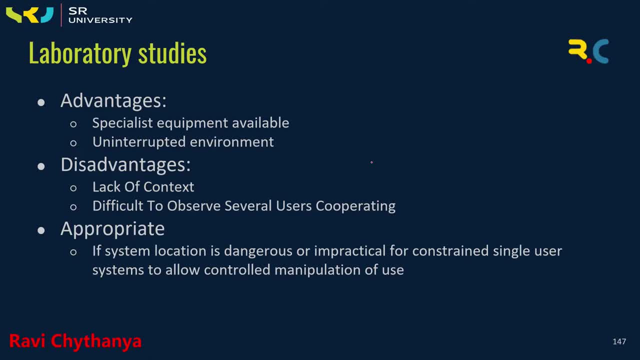 to have here advantages- okay so, and disadvantages and appropriate scenarios for the laboratory studies have been designed, discussed here. okay, the advantages are laboratory studies, are specialist equipment available and uninterrupted environment actually. so already there is an equipment to test for the, to test for the design successfully, or usability or functionality. 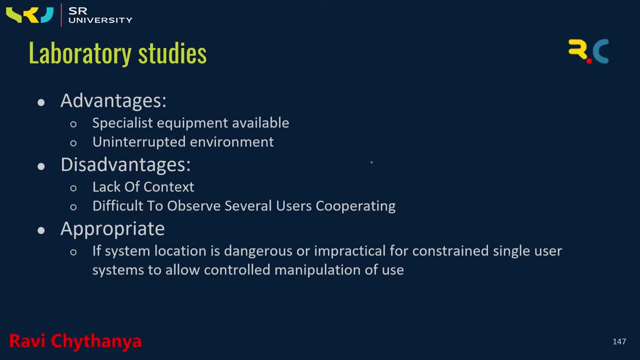 okay, so we have some equipment over there and that equipment will be used to test for the evaluate the design, and it is an uninterrupted environment. and actually there are so many disadvantages, and two of them are lack of context and difficult to observe several users cooperating, so it is. 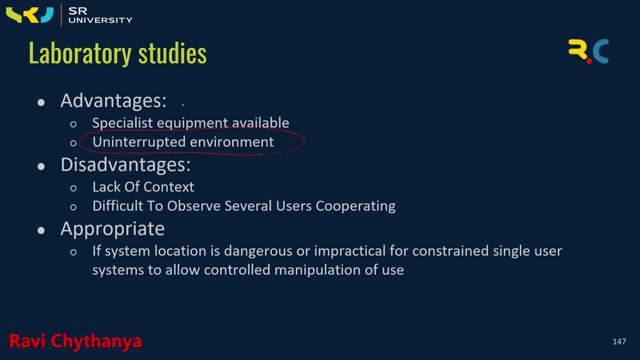 an interrupted environment and it is a laboratory. okay, so there are only one or two or more ten members of the users will be there in the study and that there it is very difficult to observe the several users cooperating with each other to give the input for the system, and it is actually appropriate. 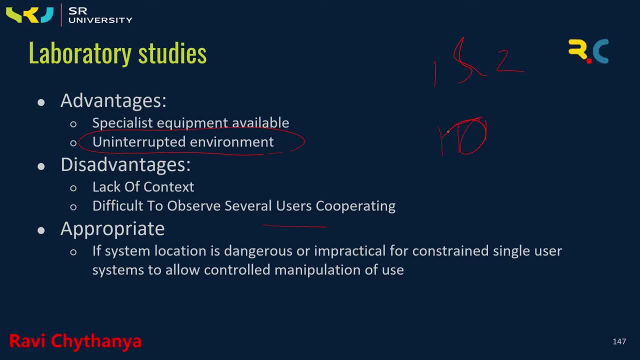 for the system appropriate for the locations. okay, the system location is dangerous because of this location is dangerous, dangerous or impractical for constrained using the user systems to allow controlled manipulation of the user. yeah, okay, so here the location actually is dangerous. okay, when the system has need to. 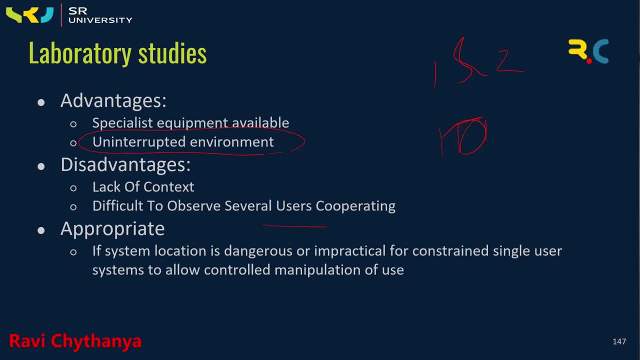 be implemented or it is, it needs to be deployed in a dangerous situation. there no need to go for clear and taking the use of other users and we need not worry about the considerations have to be satisfied. that requirement have to be satisfied or not. we are not necessary to do all the things. 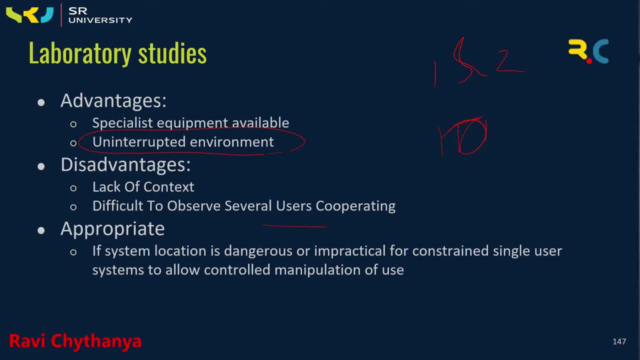 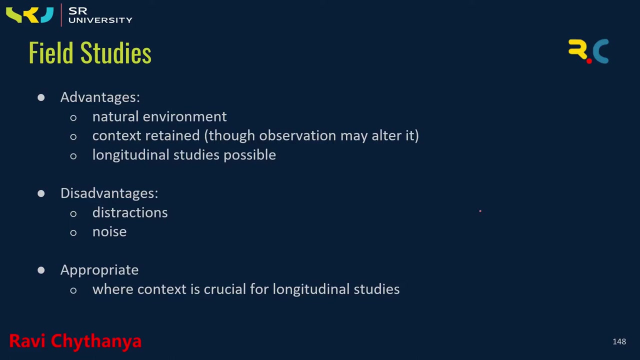 and the same situation, the same environment has been created here in the laboratory and we can go for the study and it will be very optimal, optimal for the such cases. the laboratory studies will be optimal for such cases. and then we are going to have here the field study. okay, so here you are going to, you are going to visit some field. 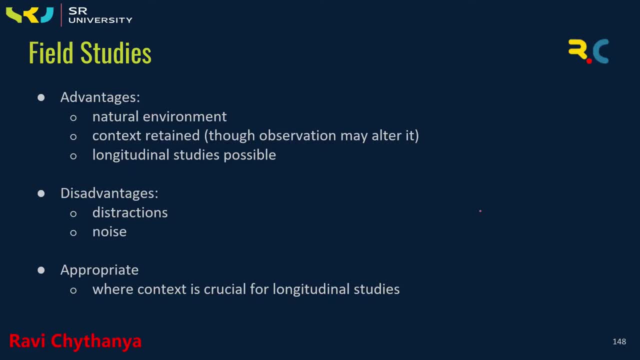 okay, and there you are going to do some studies. and if there is, if there is problem there is problem, then we are going to rectify those problems. otherwise there is no need to worry about that thing. okay, and the advantage of the field study are natural environment actually. 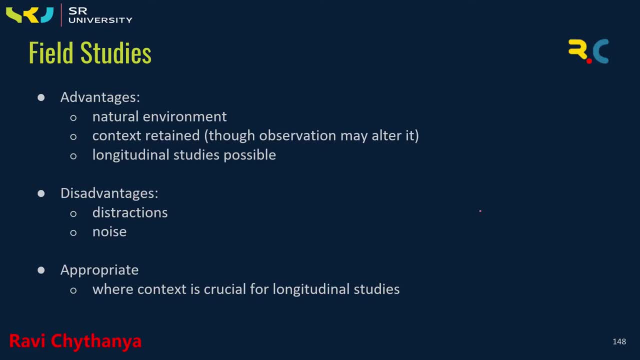 where exactly the system has to be deployed there. you are going to deploy the system for the testing purpose and that will be evaluated for the flaws in the design and the context retained. the context is going to be available with us. okay, where exactly it has to be available? where exactly it has to be available there, we are going to check for the flaws and the. 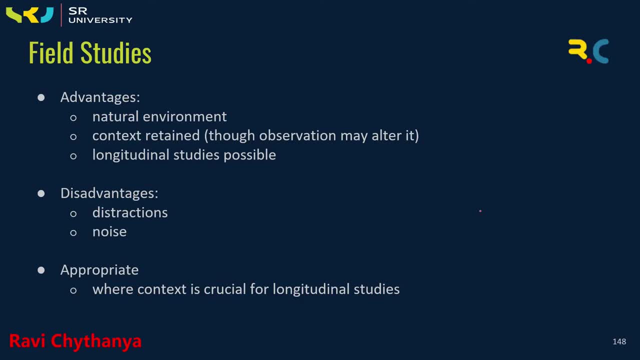 longitudinal studies possible. okay, obviously you are going to have some where you are going to. location based studies are going to be possible in the field study and the disadvantages are like, as we know, distractions and the noise will be the most- uh, optimal disadvantage for the field study. 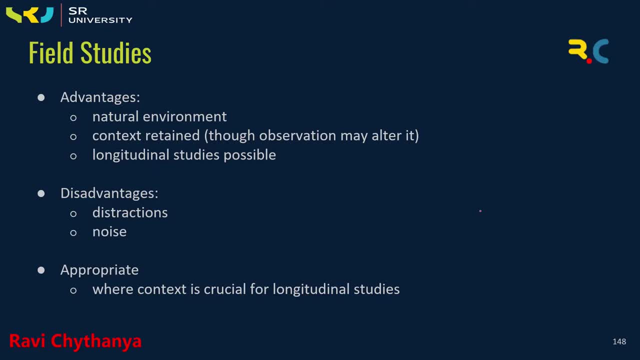 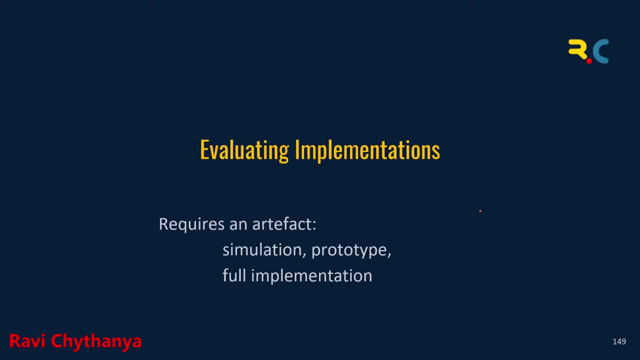 and the appropriate situation where the context is crucial for the longitudinal studies: okay. so there you can go. for the field studies, okay. and evaluating implementations: okay, so here you are going to implement. you are going to have the evaluation in terms of the implementation. so you are going to have었습니다. ok, so experimental evaluation, you are going to have the. 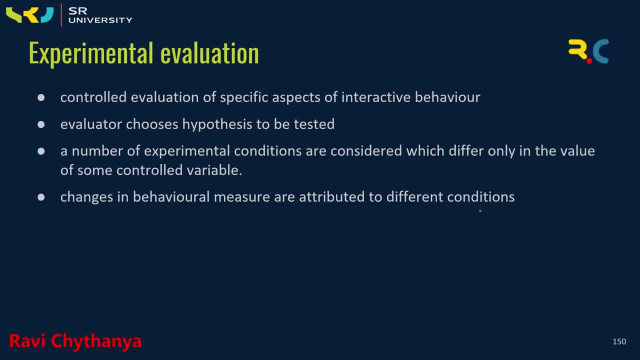 gece mishra, in which you are going to have the implementation. okay, so traditional knowledge and experience and active facts and simulation. you are going to have prototype. you are going to have full implementation you are going to have. okay, so, experimental evaluation you are going to have. 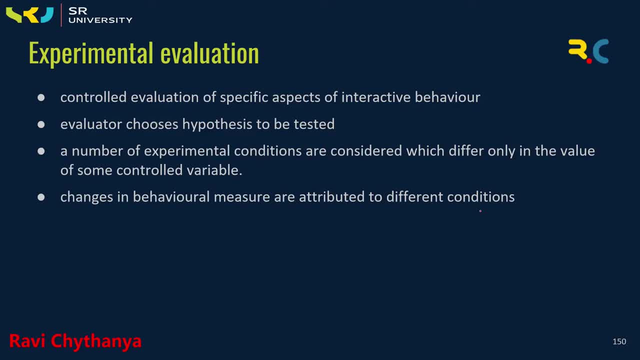 control, evolution of specific aspects of the interactive behavior. so you are going to evaluate in terms of the experiments, okay, the hypothesis you are going to have. Okay, so your way, you are going to work on the system in real time and you are going to evaluate the system for the flaws or the problems in the design. 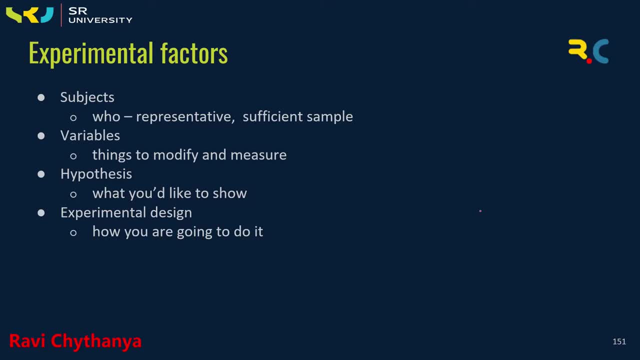 Okay, and the experimental factors are here, the subjects, variables, hypothesis and experimental design. The subjects are: who actually, who are going to participate into the experiment, and the variables the things to modify and measure actually. So what exactly you need to modify and you need to measure and you need to consider for the evaluation. 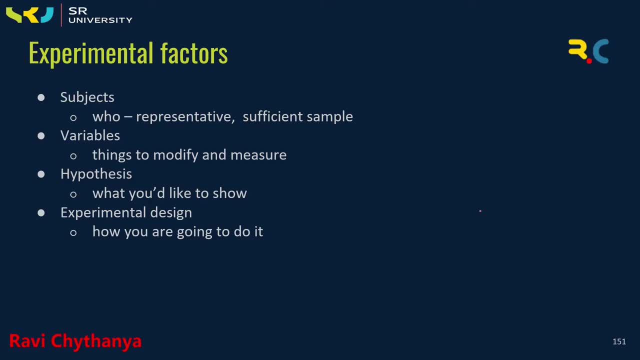 And the hypothesis, what you would like to show to the user or someone else who is actually need to use that application in the real Life or real time, and the experimental design. you are going to have some design which is going to provide how that experiment is going to be done by you. 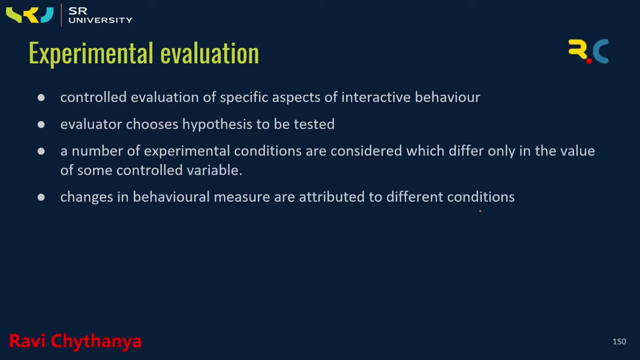 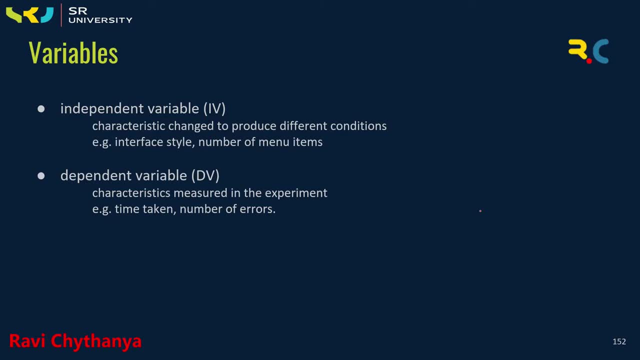 Okay, so these are the factors for the experimental evolution and the variables. here We are going to have two types of variables. One is independent variable and the dependent variable. So independent variable is nothing, but it is going to be. It is going to be observable on its own characteristic change to produce different conditions, interface style, number of main items and all these things. 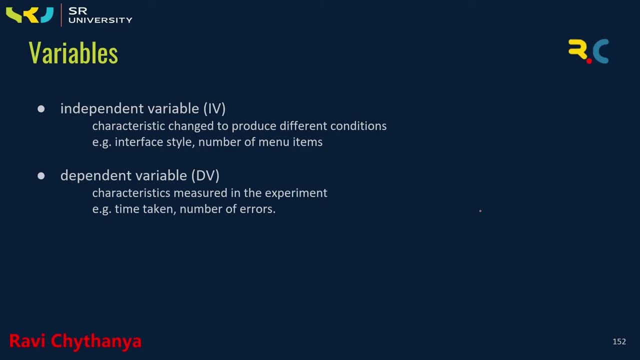 And dependent. it is going to measure in the experiment the time taken, the number of errors, the number of the usability, the usability measure and the functionality of the system. And all these are the dependent variables and these independent variables And the dependent variables are going to be evaluated in the experimental evaluation. 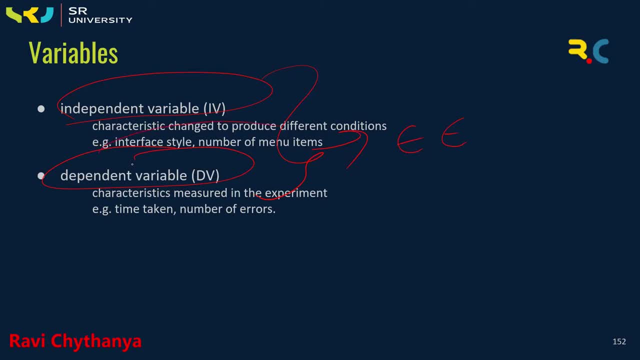 Experimental evaluation, And this is going to be called as the functionality And this is going to be called as the usability. Okay, so the independent variables are going to provide the functionality of the system and the dependent variables are going to provide the usability of the system. 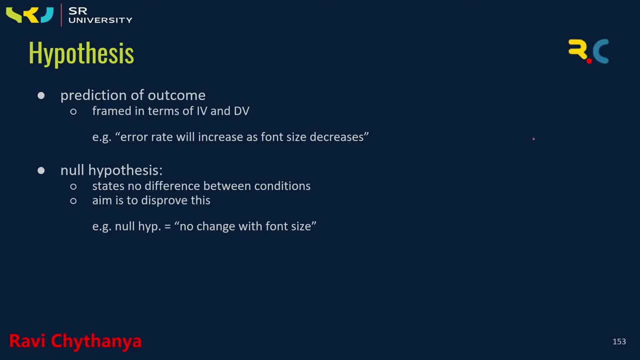 And the hypothesis is going to be prediction of the outcome- What exactly the outcome has to come first. we are going to predict And, if it is, that is going to be framed in terms of the independent, independent variables as well as the dependent variables. 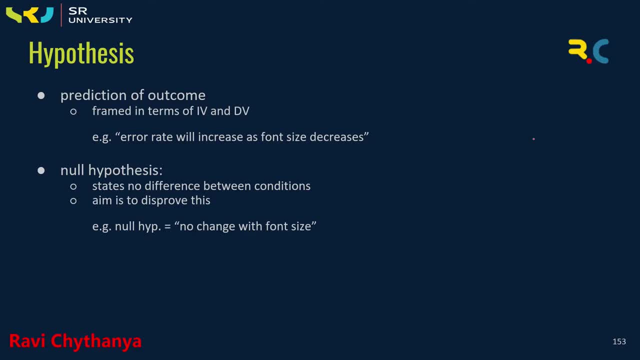 And the- And the example here is error rate will increase as font size decreases. obviously, if i am going to decrease the size of the font, okay, then the usability, the visibility of the screen, the visibility of the questions are, the visibility of the interface is going to be reduced and the 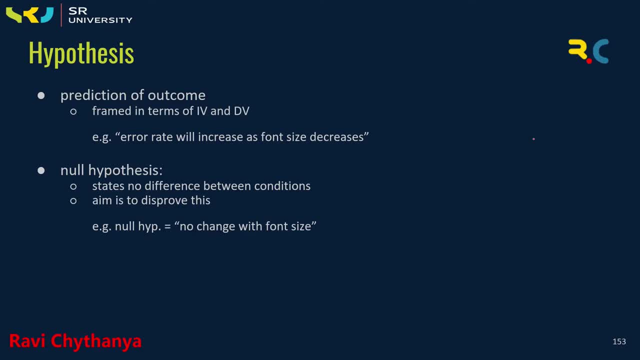 errors will be increasing and we are going to have the null hypothesis. it is going to states no difference between the conditions and aim is to disprove this. null hypothesis is equal to no change with the font size. actually, this is a wrong statement. the hypothesis should be provided. 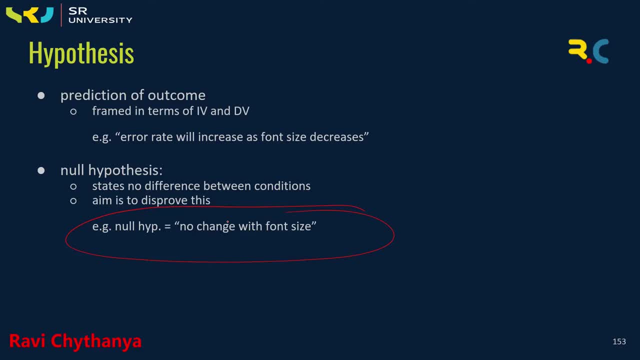 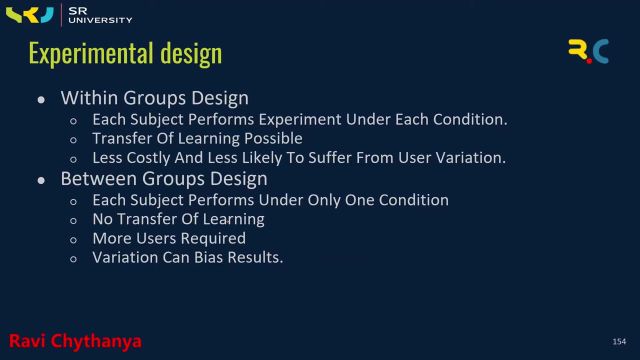 for such that the, whatever the conditions you are going to satisfy, you need to satisfy, they need to be satisfied based on the based on the systems inter independent variables and the dependent variables and the experimental design. here you are going to have the within the groups and between the. 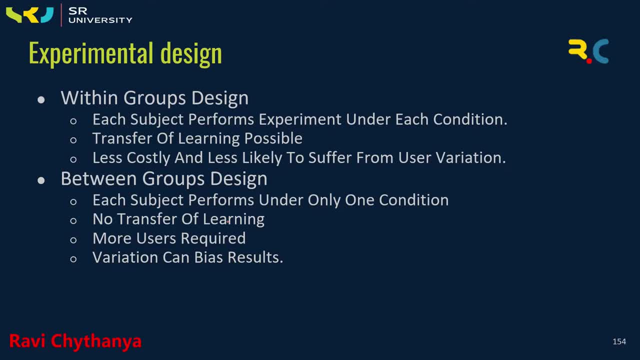 groups: you are going to have experimental design within the group's design. each subject performs experiment under each condition. transfer of learning possible, less costly and less likely to suffer from user variation. and between groups design: you are going to have each subject to. each subject performs under only one condition and no transfer of learning and more user. 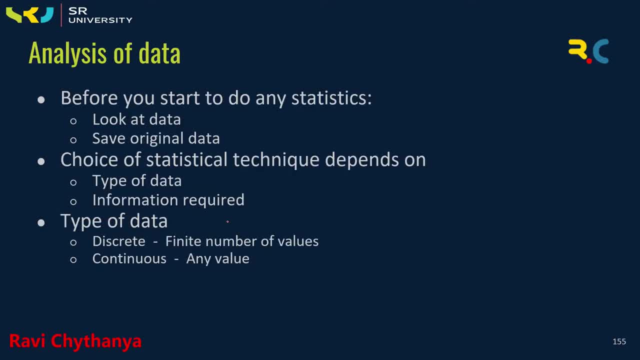 required variation can be biased. results: okay, and the analysis of the data. before you start to do any statistics, you need to look at the data and you need to save the virtual data and work on the copied data. otherwise the original data will be replaced by the modifications or the 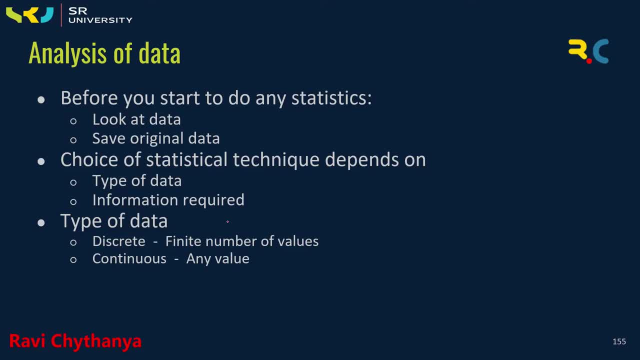 characteristic heuristics we are going to take into the consideration for the evaluation and the data is not going to be replaced. the data is not going to be replaced. it will be replaced by the re placed or regained from the to the original data and the choice of the statistical techniques. 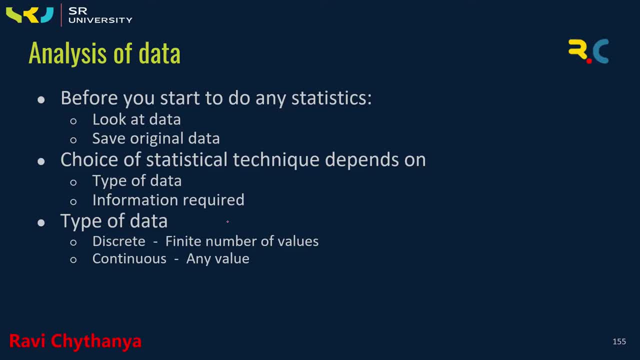 depend depends on the type of the data and the information we required to evaluate the system. and the type of data will be of two types: discrete and continuous. the discrete is nothing but finite number of values and the continuous any number of the values you are going to have. okay, and the 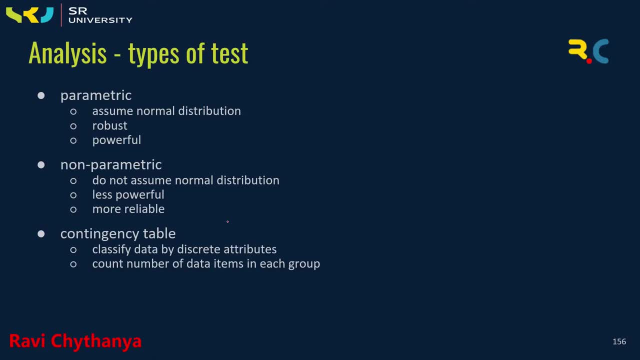 analysis. here you are going to have the types of the tester. the first one is parametric, the second one is non-parametric and third one is contingency table. the parametric is nothing but assume normal distribution. robust and powerful you are going to have, and non-parametric it is going to. it is 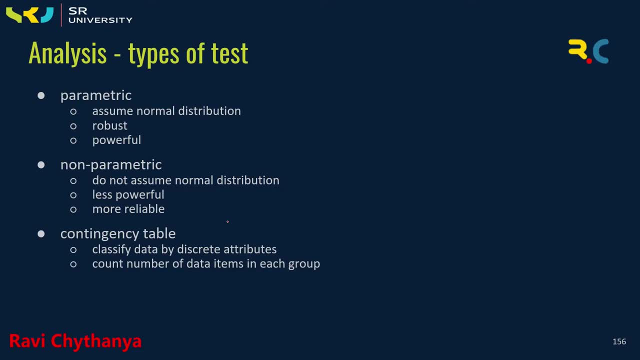 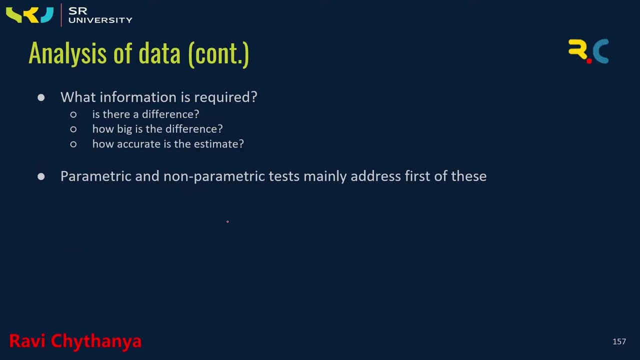 not going. it doesn't assume normal distribution of the data and it is less powerful actually and but less powerful but it is more reliable and the contingency table it. you are going to classify the data by the district- discrete attributes, okay- and count number of data items in each group. you are going to and the what information actually you need to. you require for 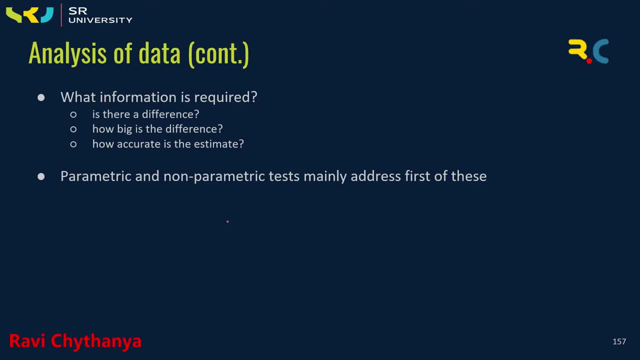 the analysis of the data. is there any difference? first one, and if there is any difference, then how big is the difference? and then, if the big, biggest of the difference you are going to have, then how accurate is the estimate? how accurate, whatever you estimated? okay, how accurate is the estimate? and here the 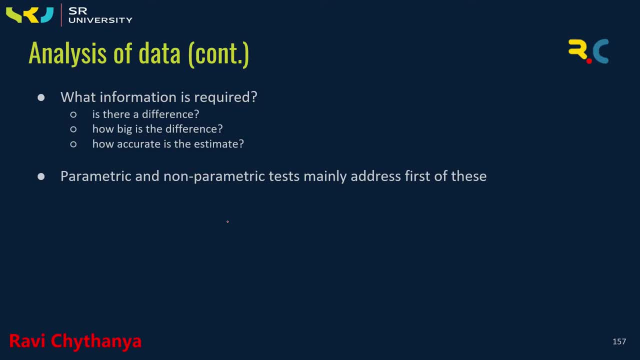 difference between the estimation and the exact values. analysis of the data. output of the outcome of the analysis of the data. if there is any difference, then how big is the difference? and, uh, how accurate is the estimates? if the difference is small, then the accuracy will be high. 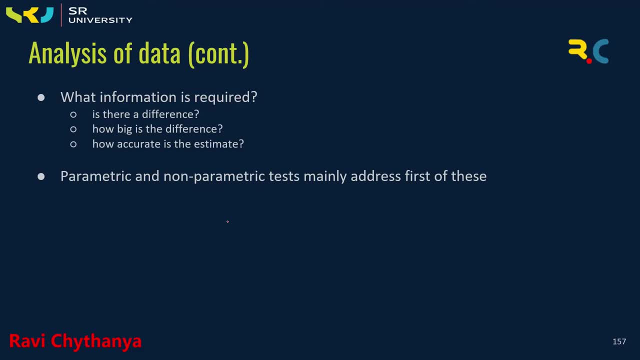 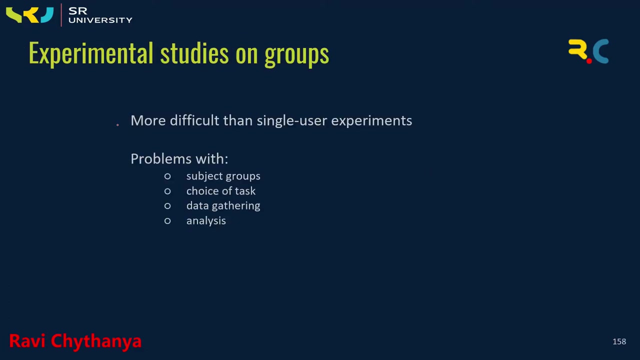 and the parametric and nanoparametric tests. mainly address the first of these parametric and nanoparametric are going to be and addresses the. addresses the difference between the estimated and original data and experimental studies on groups- okay, this is actually in the groups and this is on groups. okay, more difficult than single user experiment and the problems with 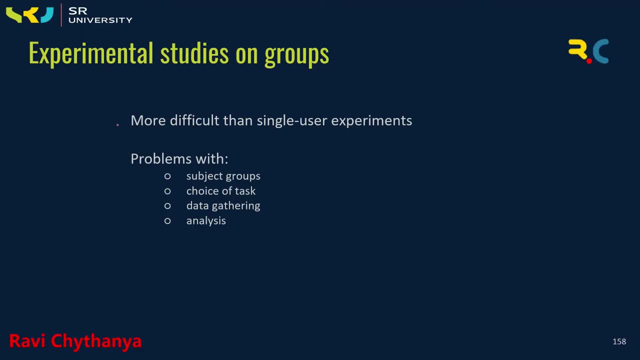 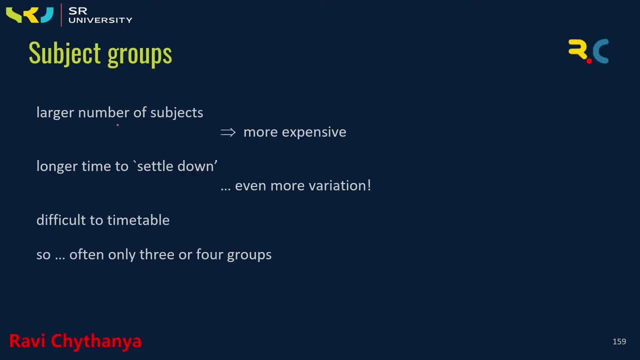 the subject groups, choice of task, data gathering and analysis. okay, so next subject groups. here you are going to have now larger number of subjects, more expensive, it will be longer time to settle down, even more variation, difficult to timetable, so often only these four groups. you are going to have actually larger number of the subjects. if you are going to have, then it will be. 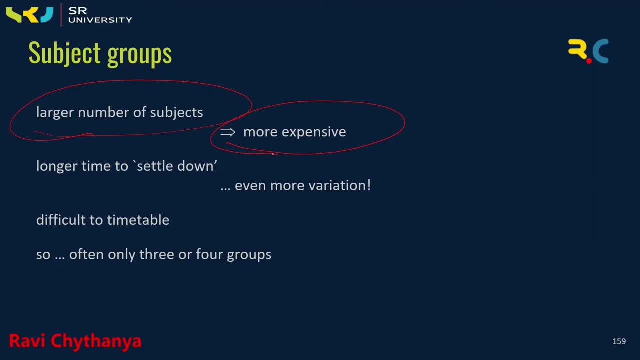 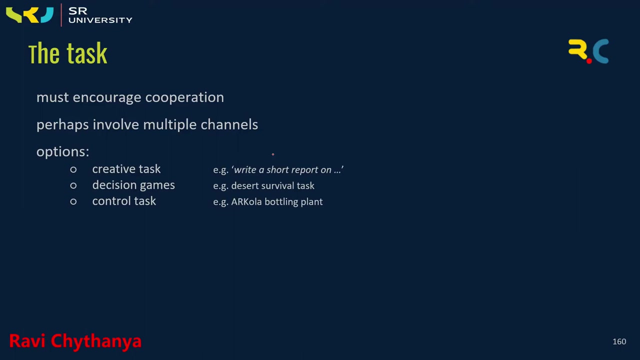 more expensive and longer time it is going to settle down. okay, so you are going to have the more variation and it is actually difficult to the time table and the task is here we are discussing about the task, task, task. here it is going to encourage the cooperation, the task, and it perhaps 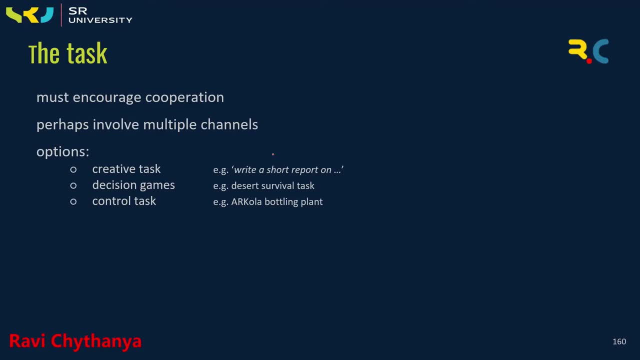 involve the multiple channels, multiple users into this task and the options we have for the task are okay: creative task, decision game control task. the creative task example is: write a short report on something, something, something. you are going to have, a creative task which is going to, which is: 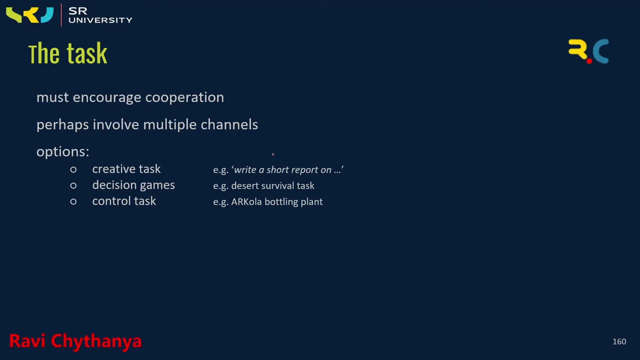 going to ask you for writing a short report on the some task you have given and the decision games task you are going to give with some task- desert survival. so you are going to decision based on the survival of the survival of yourself in the desert and the control task is nothing but our. 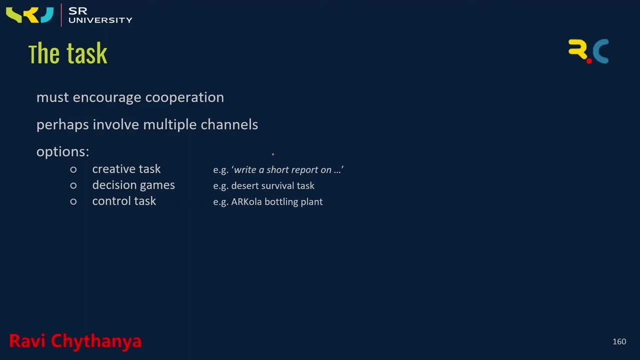 cola bottling planche it is going to have. so these are the different tasks we are going to have and these tasks must encourage the cooperation among the users and the data gathering. okay, so the data will be gathered through several video cameras, so the data gathering is a direct logging of application and the problem is problems with. 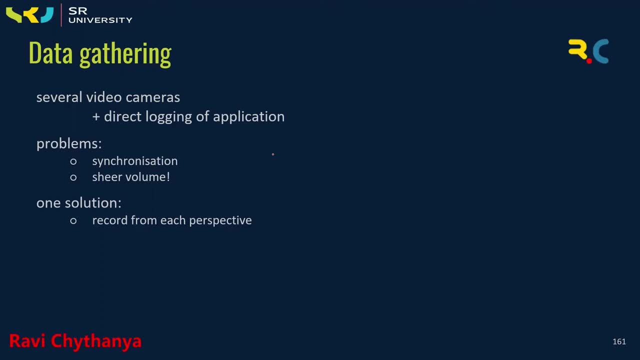 the data gathering are synchronization and shear volume, and the one solution is record from each perspective. so if you are going to have a room, okay, and if you want to record all the data, save the save the data from this room, okay, then you need to record from all the eight perspectives. 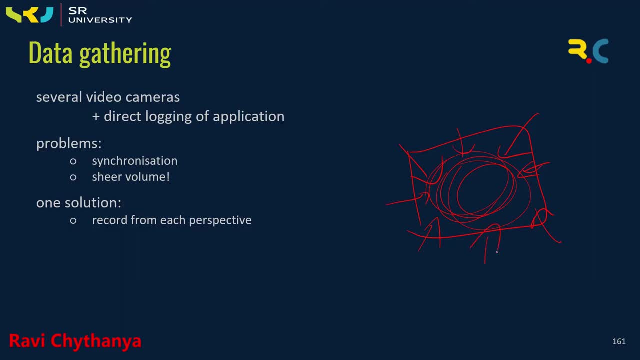 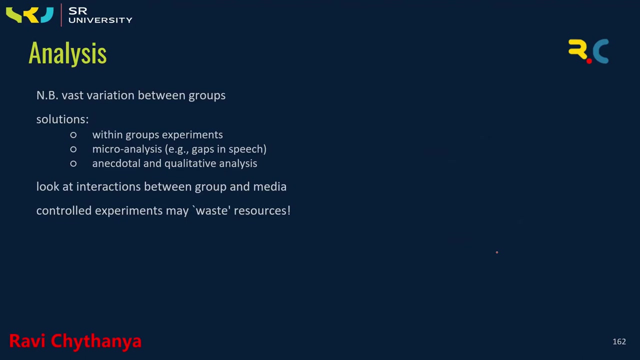 this is an example only. so, from each perspective, you need to record and the perfection based on the perception, the based on the perspective, you need to consider which one has to be taken into the consideration, into the consideration and the analysis of the data gathered will be vast variation between the groups and the solutions for the vast variation is 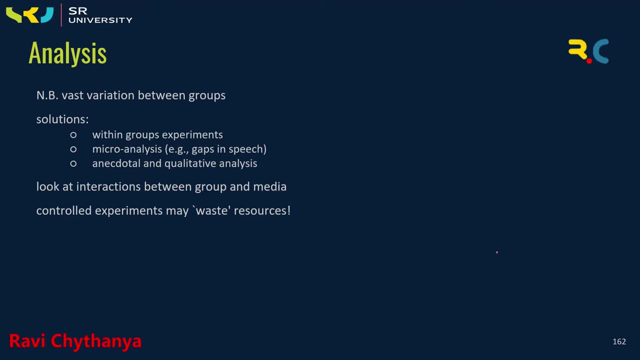 within group experiments you need to do and micro analysis you need to have. the gaps in between the speech and anecdotal and qualitative analysis you need to perform and the look at the interactions between group and media. unit 2, 2 and controlled experiments may waste the resources. this is regarding the. this is regarding 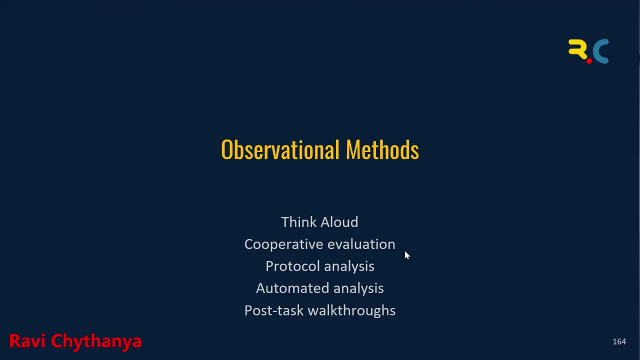 the analysis of the data. okay, next we are going to discuss about the observational methods. we are going to call this one as actually the classification of the classification of the evaluation. okay, so the classification is: think, allowed, cooperative evaluation, protocol analysis and automated analysis and post-task walkthroughs you are going to have and we are going to learn about these. 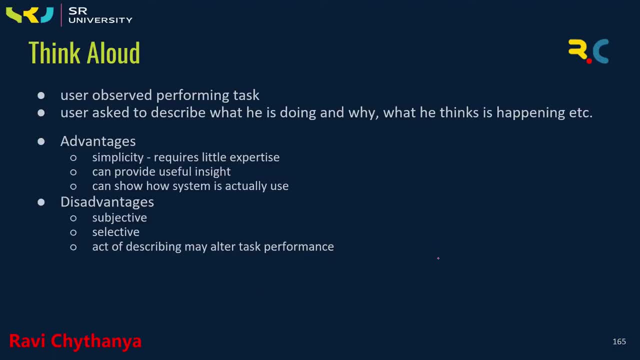 five types of the classifications of the evaluation: okay, the think allowed. user observed: performing task in the think allowed. okay, so the user is going to be observed for the performing of the task. okay, and user as scripture to describe what he is doing and why, what he thinks is happening, etc. so here, 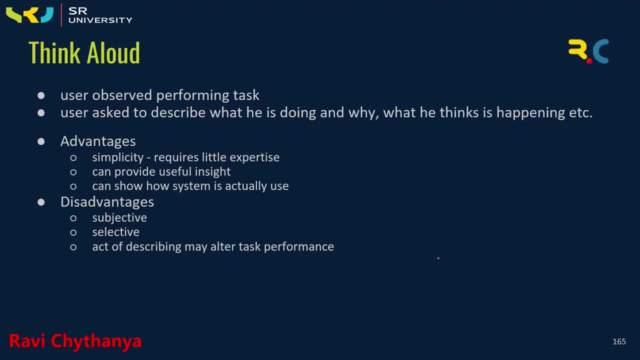 in the tall think allowed evaluation technique, the user is going to be concentrated, okay, and the user is going to be asked to describe what actually he is doing and why he is doing and what he thinks is happening when he is going to do something. the advantages of the think allowed are: simplicity, can provide. 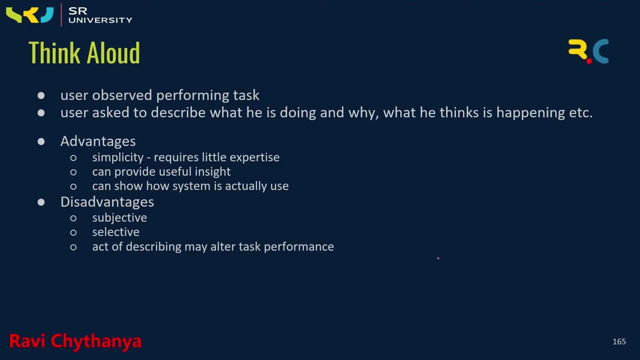 useful insight and can show how system is actually used. because because the user here writing or describing what exactly he is doing with the system and the disadvantage of the thing color are actually the subject. you, okay, it is going to be subjective, and select you because it is going to be based. 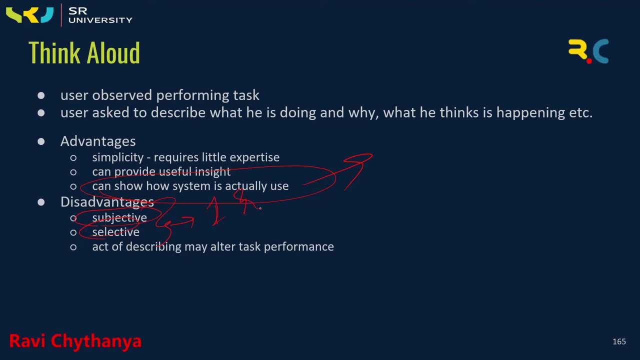 on what is being said and not what is being said, and it is going to be based on on only one or a limited number of users, and then users are going to have- may have our own, just like us, and art of describing may alter task performance. okay, so the describing is going to alter the task performance option because he 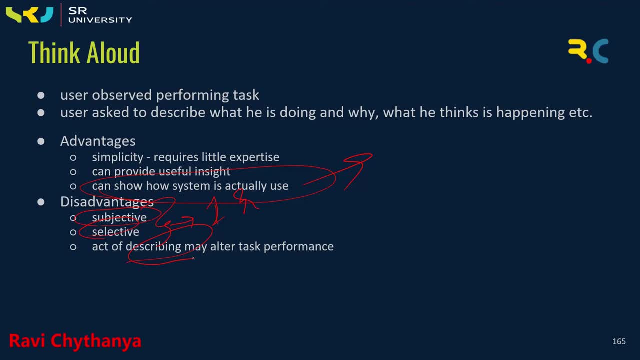 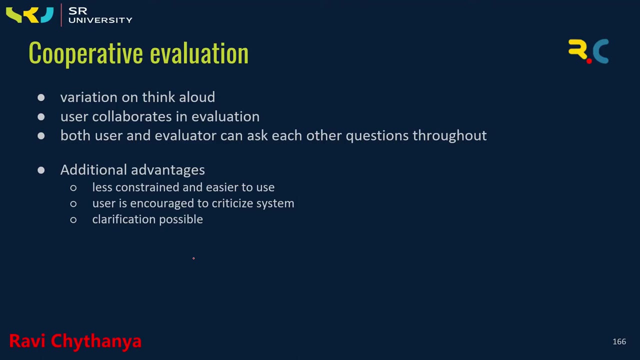 is going to concentrate on the describing only. he is not going to use the actual, he is not going to perform the task in an fully concentrated way. so this is the first one, the think allowed, and the next one is cooperative evaluation. here variation is going to be on the think allowed the user. 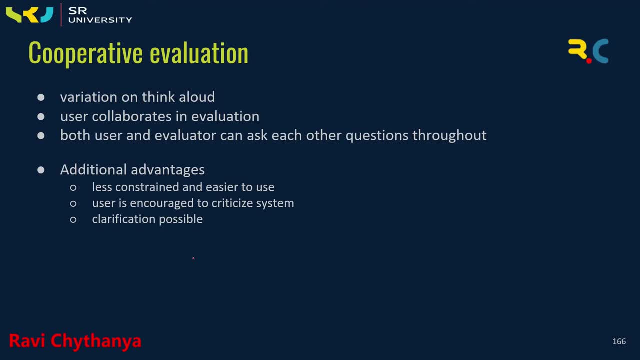 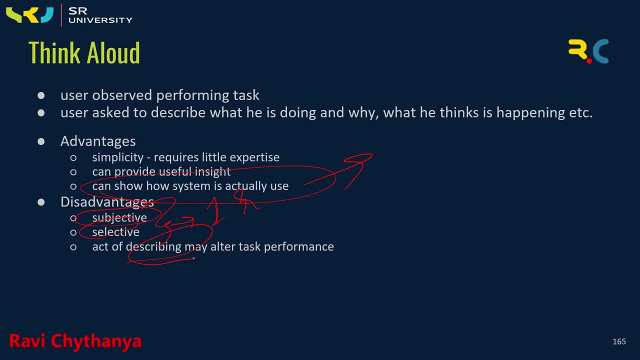 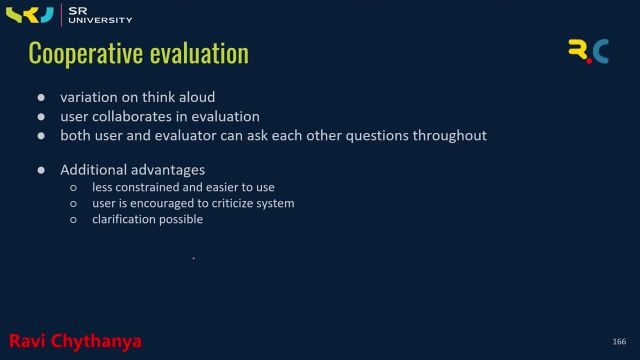 collaborates in evaluation. both user and evaluator can ask each other questions throughout here. in the previous think aloud, the user only is going to be participated into the evaluation process and in the next one, cooperative evolution, the user as well as the evaluator are going to be participated into the participated into the. 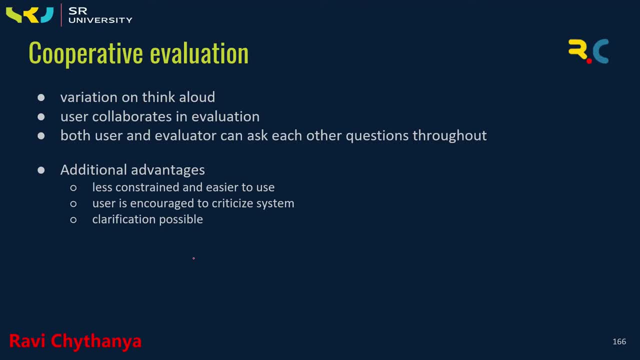 evaluation process and they are going to ask each other questions throughout the task. performance and the advantage. additional advantage is, along with the think, aloud, less constrained and easier to use. user is encouraged to create this system. and going to be possible because here the evaluator is also participating in the system evaluation. 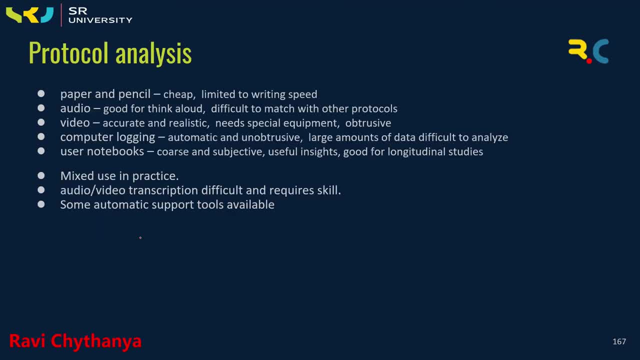 okay, and next one is protocol analysis. it is a paper and pencil based- okay, so it is very cheap, limited to writing speed and if you are going to have audio, good for think aloud, difficult to match with other protocols, and if it is belongs to video, it is accurate and realistic. needs special: 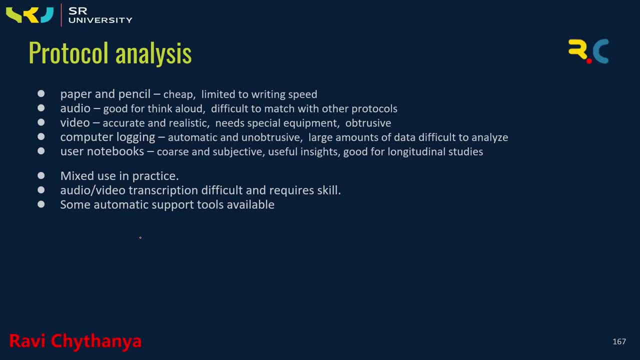 equipment like cameras and the lighting and all these things and it is obtrusive. and the computer logging. actually you are going to have automatic and unobtrusive large amount of data difficult to analyze. so the logging is nothing, but it is going to make some note into somewhere else. 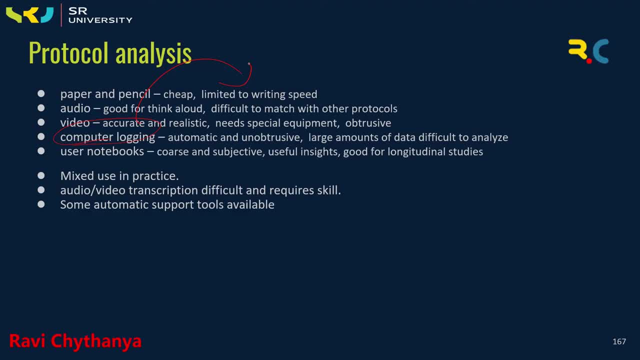 whatever you are going to do, and the user notebooks- actually this is going to happen, course- and the subjective, useful insights, good for language tutorials, and this is going to be protocol analysis is going to be used with mixed use in practice, either with the audio video or video computer logging or audio computer logging or something, something audio. 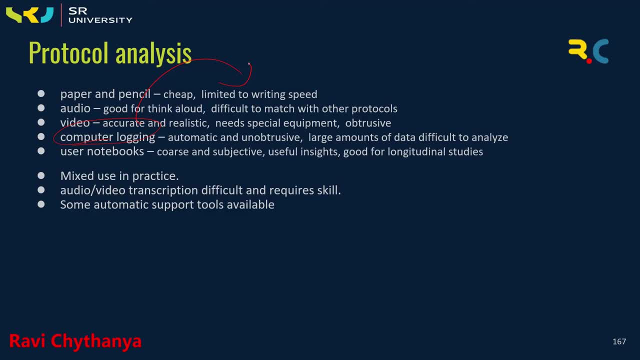 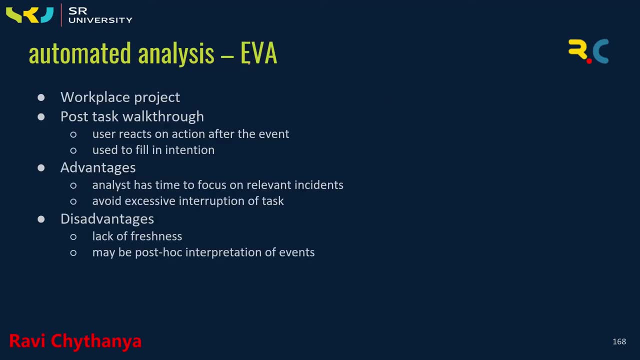 video transcription difficult and request skill and some automatic support tools are available for the audio video transcription. okay, so then automated analysis, eva you are going to have here. so workplace project it is, i think actually- and post task walkthrough will be there. user reacts on action after the event. user use it. 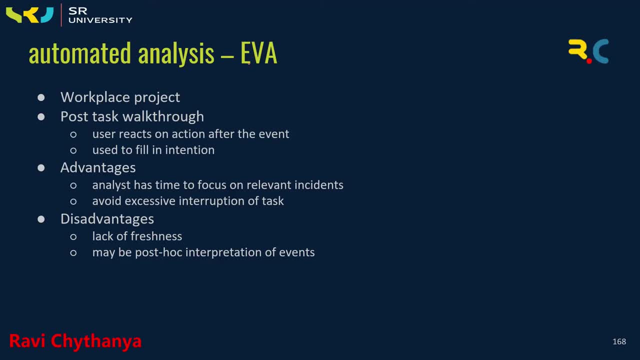 to fill an in intention. you are going to have some form, feedback form after using of the task, after performing of the task, and that has to be filled in intention. and the advantage with the automated analysis is analyst has time to focus on relevant incidents and avoid excessive interest interruption. 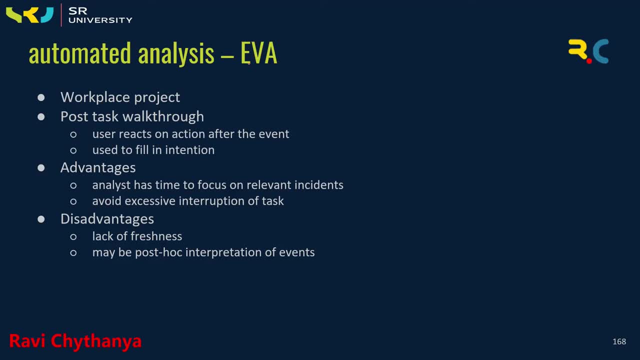 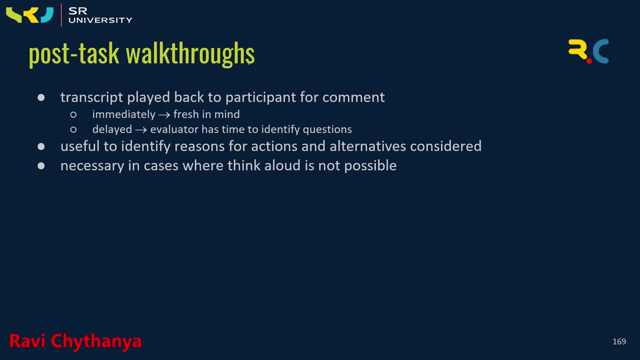 of the task. the advantage of the automated analysis are lack of freshness and maybe post hawk interpretation of the events. okay, and then post talk was post task walkthroughs. okay, already i have told you task. after completion of the task you are going to have some walkthrough, some. 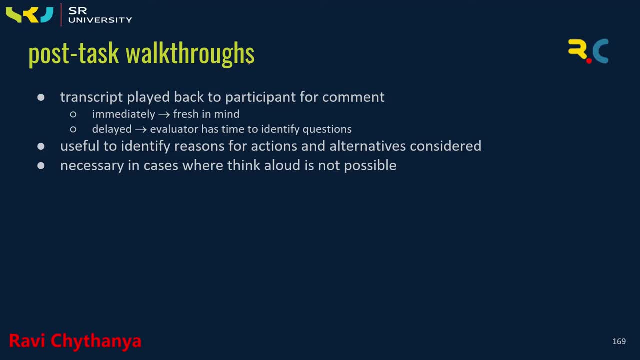 feedback or some filling forms are going to be given and the transcript played back to participant for comment immediately, fresh in mind. delayed evaluator has time to identify the questions. it is useful to identify regions for actions and alternatives considered. so it is used to identify the reasons for actions and alternatives considered unnecessary in cases when Tinkuent is not possible. 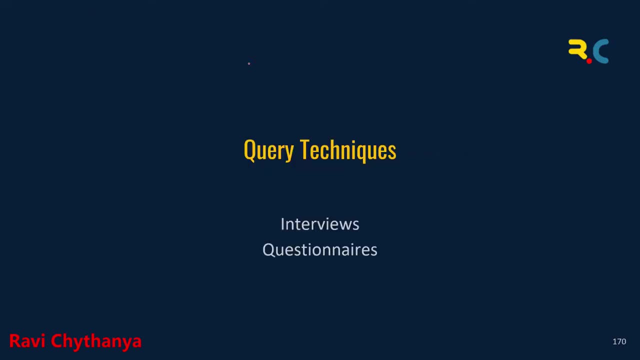 okay, so this is regarding the first task box Force, and these all are the different types of the classification of the evaluations. okay, observational methods, queries. and in the observational methods you are going to have the think aloud, cooperative evolution, protocol analysis, automated analysis, post track, post to task workflows. and then the next classification of the classification of 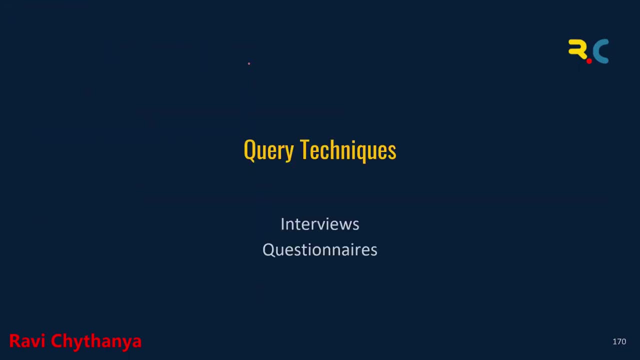 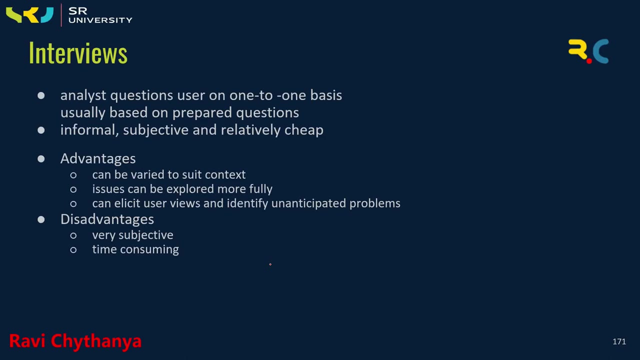 the evaluation is going to have the query techniques. here you are going to have the interviews and the some questionnaires and the interviews analyzed. questions: user on one-to-one basis, usually based on prepared questions, obviously, and informal, subjective and relatively cheap. so after completion of the using of the performing of the task, the user has to answer some questions. 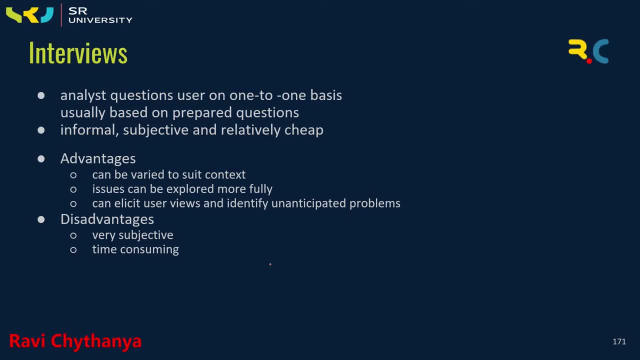 prepared questions: okay, and the advantages of the interviews are: can be varied to suit context. okay, so one user is using in one context, another user is using another context. okay, in the previous, the post task walkthrough or the automated, automated analysis or whatever you have learned in the previous one. okay, those. 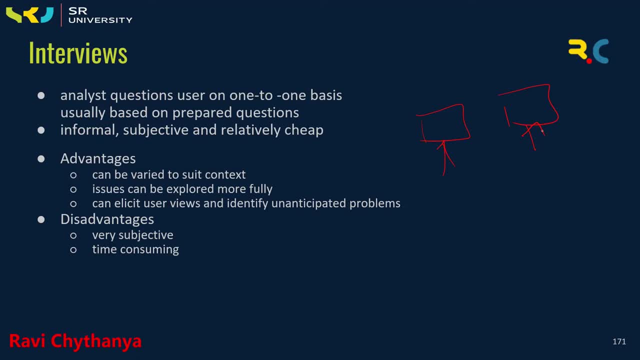 are actually with a for every context. the question is: the analysis will be the same, but here in interview, okay, the user is going to the questionnaire, the evaluator is going to ask the questions after completing of the performing of the task, based on his context, and issues can be explored more fully. and 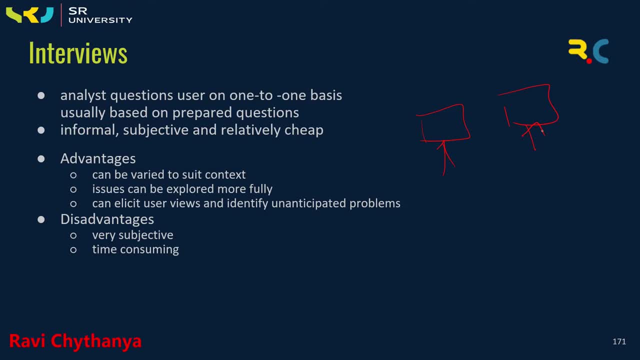 can elicit a user views and identify unanticipated problems it is going to have, and the disadvantage is very subjective and time-consuming, actually, because for every user I need to ask, I need to prepare some questions and I need to ask, ask the questions and I need to get the feedback from them and then I 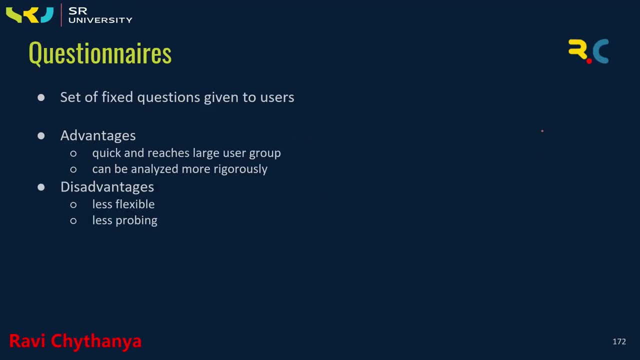 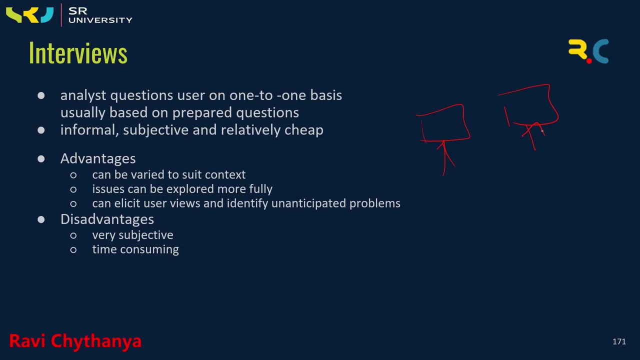 need to evaluate so it is time-consuming and the questionnaire- set of questions, set of fixed questions given to users and quick and reaches large user groups- can be analyzed more rigorously. and less flexible, less probing and it is actually the the. it is not suited for the context.